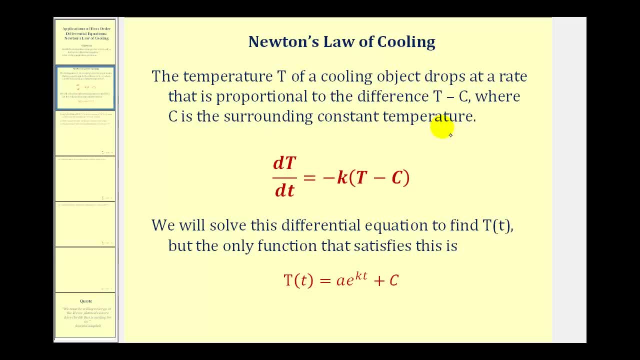 and C is the constant temperature of the surrounding environment. We can express this as dT. dt equals negative K times T minus C. This is telling us the change in temperature with respects to time of the cooling object is equal to the opposite of a constant. 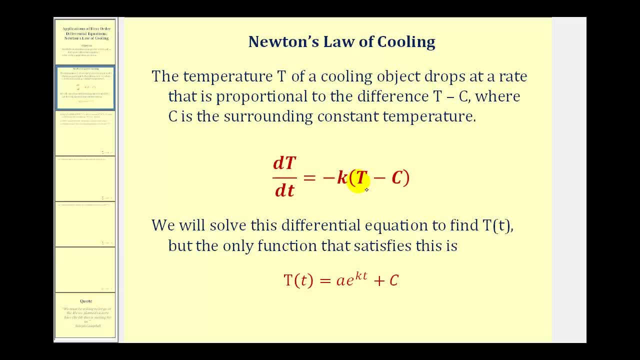 times the quantity T minus C, Again, where T is the temperature of the cooling object and C is the temperature of the surrounding environment. We will solve this differential equation to find T of T, but the only function that satisfies this differential equation or the general solution to this. 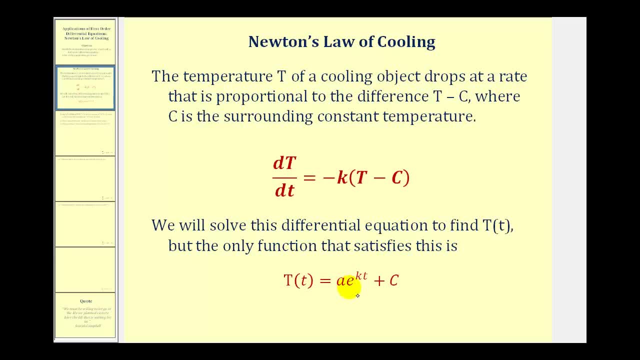 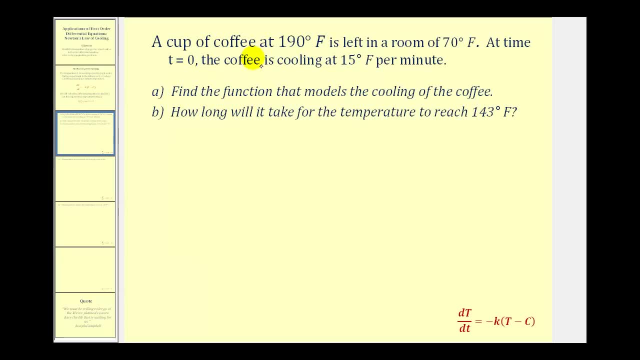 would be: T of T equals A times E raised to the power of KT plus C, And we'll discover this in our first example. A cup of coffee at 190 degrees Fahrenheit is left in a room of 70 degrees Fahrenheit, At time T equals zero. 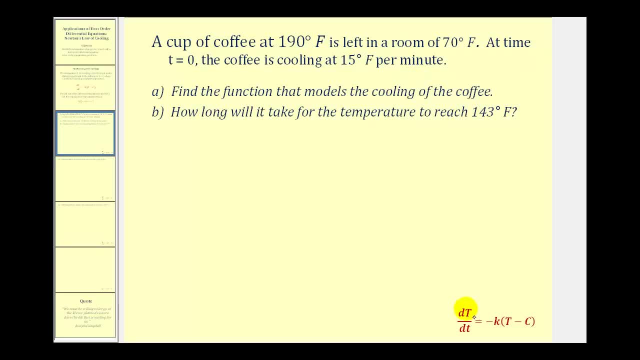 the coffee is cooling at 15 degrees Fahrenheit per minute. So, using Newton's Law of Cooling, given here below, we need to be able to recognize that dT, dt- the change in the temperature with respects to time- is equal to negative 15 degrees. 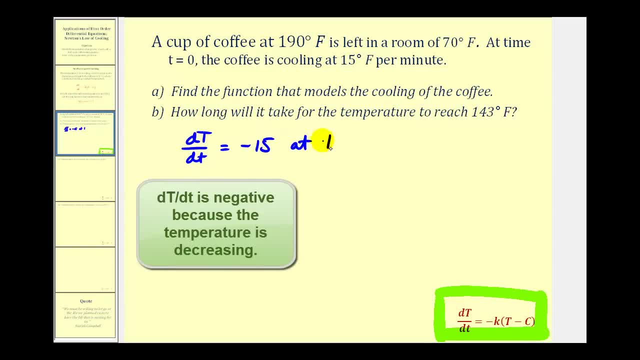 or negative. 15 at T equals zero And the coffee starts at 190 degrees. therefore, capital T is equal to 190, and capital C, or big C, is the temperature of the room, which is 70 degrees. So, using this information and Newton's Law of Cooling, 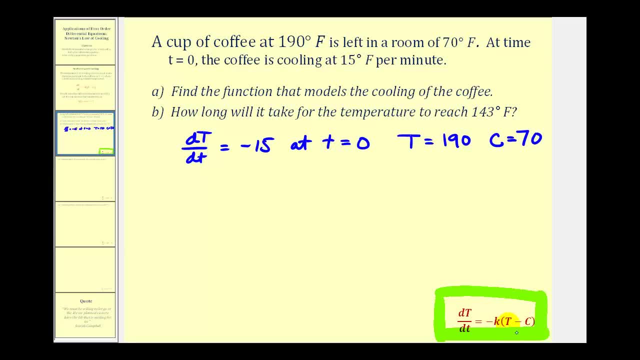 our first step is to find K by the constant of proportionality. So we want to solve the equation: negative 15 is equal to negative k times the quantity t minus c, which would be 190 minus 70. So here we have: negative 15 is equal to. 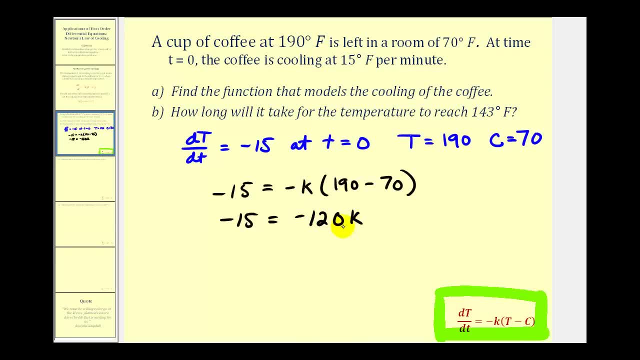 this is going to be negative 120k. Divide both sides by negative 120.. So we have: k is equal to. this simplifies nicely to 1 eighth or 0.125.. Now that we know k, we're going to substitute this value. 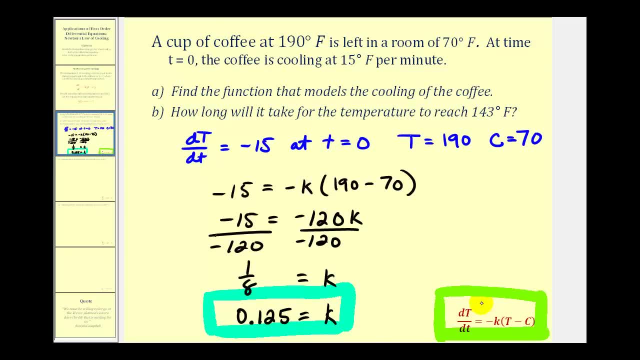 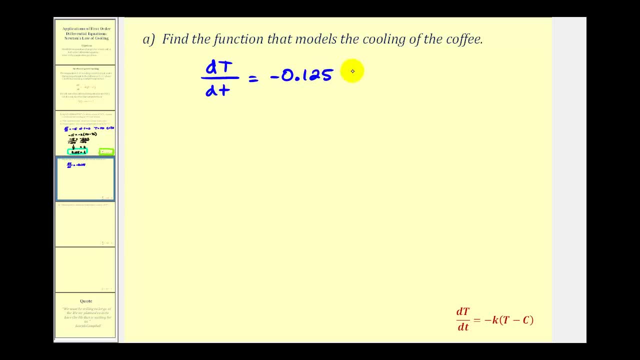 into Newton's law of cooling to solve this differential equation. So now we know dt. dt is equal to negative 0.125.. Times the quantity t minus c. We know the temperature of the room will not change, So we have t minus 70.. 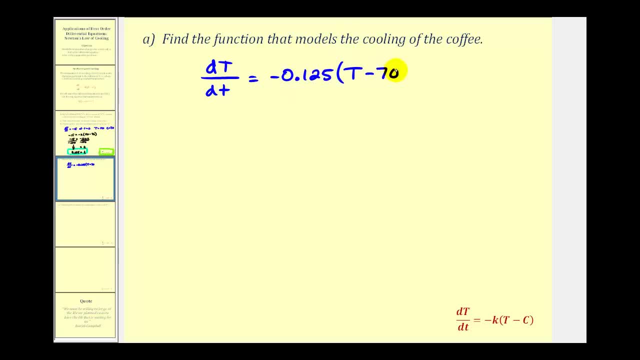 And we also know that big T of zero, the starting temperature of the coffee, is 190.. So now we can solve this as an initial value problem And we can solve this using separation of variables. So for the first step, let's write this in differential form: 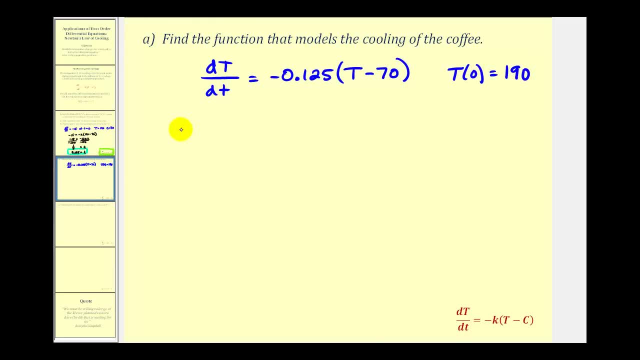 We have d of big T and we have t minus 70. So we have t minus 70.. We have t minus 70. This is equal to negative 0.125 times the quantity t minus 70, dT. And because we want big T on the left side of this equation. 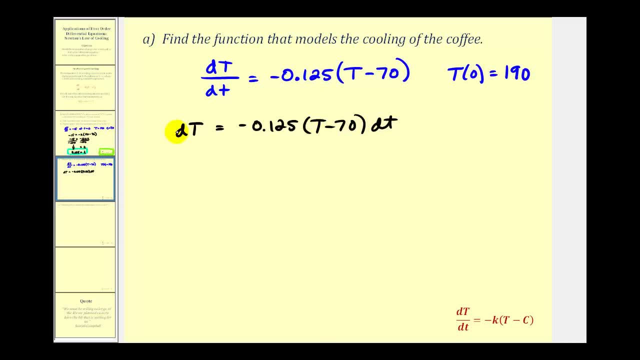 we're going to multiply by the reciprocal of t minus 70,, which would be one over t minus 70. So we have one over t minus 70, d big T is equal to negative 0.125, d big T. 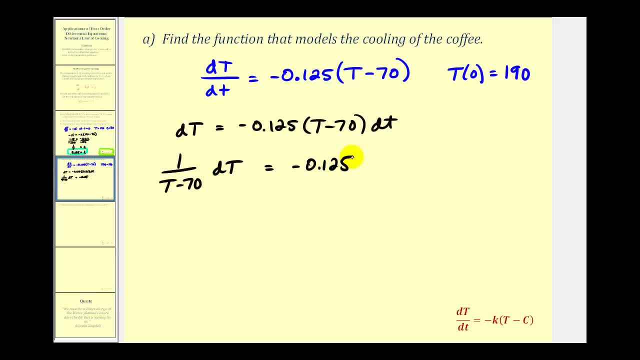 So we have one over t minus 70, d big T is equal to negative 0.125, d little t. And now from here we can integrate both sides of the equation. Our anti-derivative here is going to be: 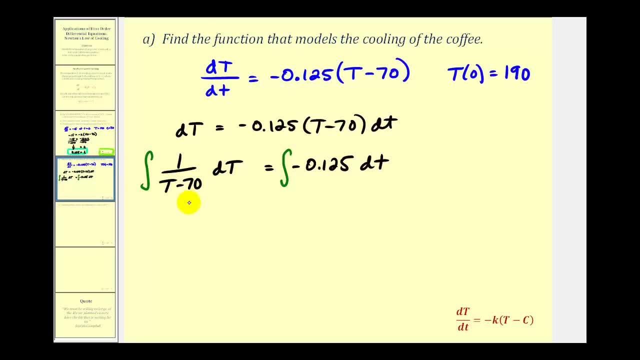 natural log: absolute value of capital: T minus 70. But we know t is never going to be less than 70, the temperature of the room, So we can leave the absolute value off. We'll have natural log of T minus 70,. 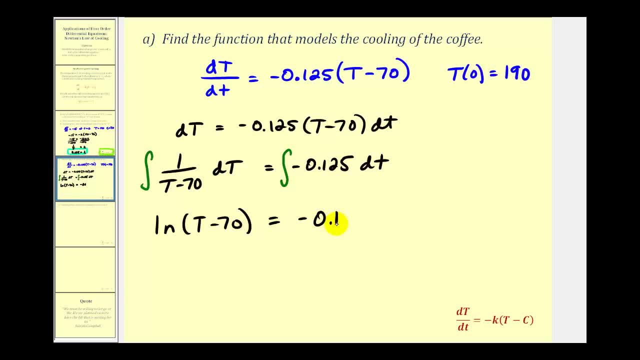 or big T minus 70, equals negative 0.125 times little t plus our constant of integration, and our goal is to solve this for big T. So if this equation is true, then e raised to the power on the left side of the equation. 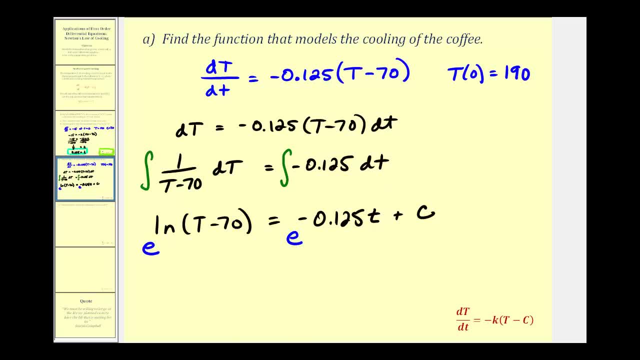 must equal e raised to the power on the right side. So the left side simplifies nicely to big: T minus 70, equals on the right side. notice how we're adding these exponents. this is the same as e raised to the power of. 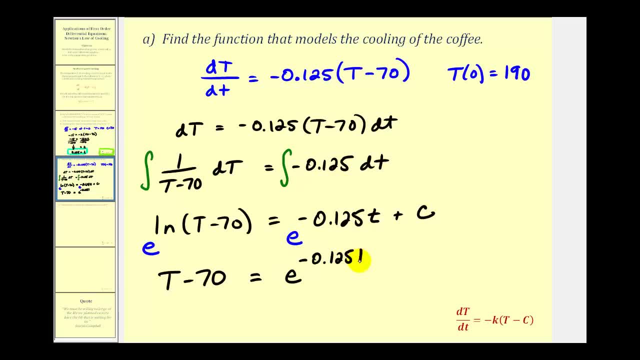 negative 0.125t times e to the c, which is equal to. well, if c is a constant, e to the power of c is also a constant. so from here we're going to let e to the c just equal a constant a. 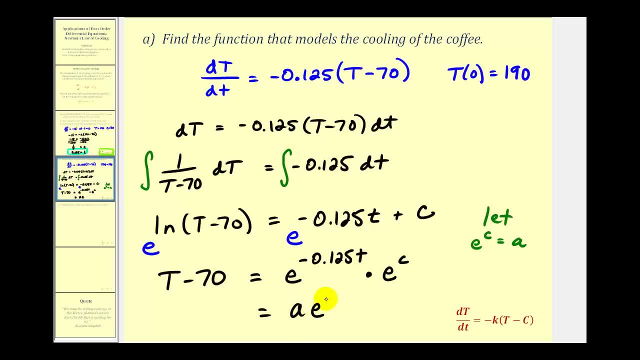 So we can write the right side as a times e to the negative 0.125t and to solve for t we're going to go ahead and add 70 to both sides, so we'll have plus 70, and because this is a function of little t, 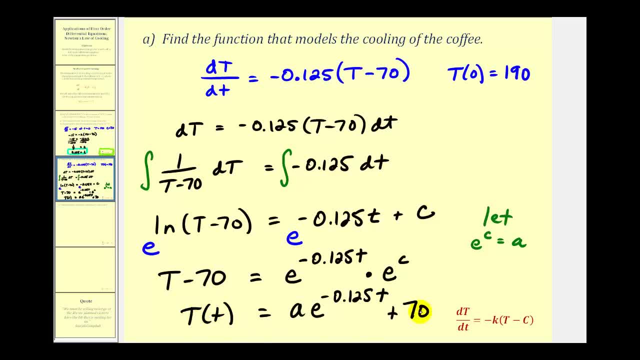 we have: big T of little t is equal to this right side. So now we can take this general solution and use the initial condition- big T of 0 equals 190, to find the value of a and find our particular solution. 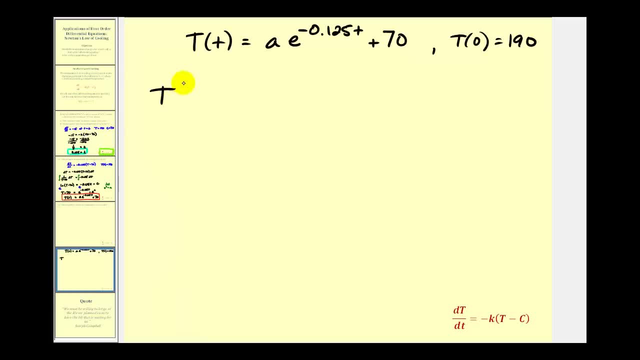 And let's do that on the next slide. So if big T of 0 is equal to 190, then we'd have a times e to the 0 power, which is just 1, plus 70, equals 190,. 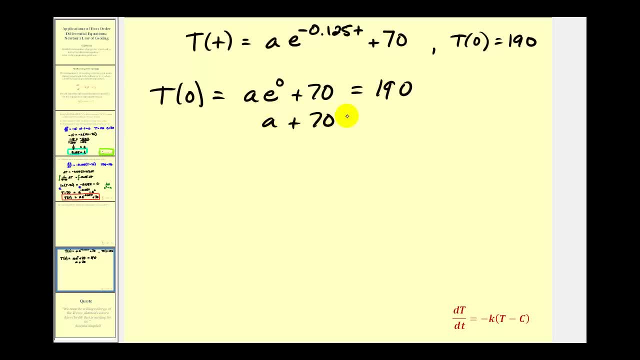 so we have a plus 70, equals 190, and so we have a equals subtracting 70 on both sides 120.. So our particular solution with a function that models the cooling of this coffee is big T of t. 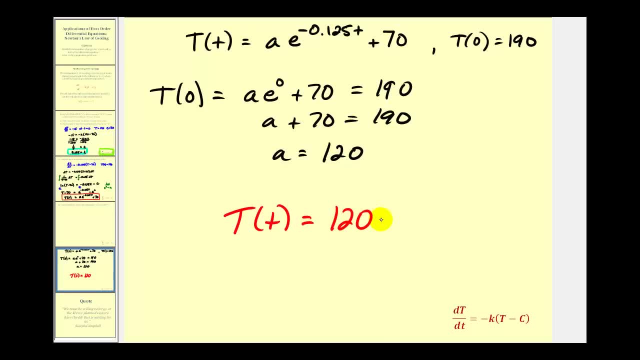 equals again: a is 120, e to the negative 0.125t plus 70.. And now we can use this function to answer the last question, which was: how long will it take for the temperature to reach 143 degrees? 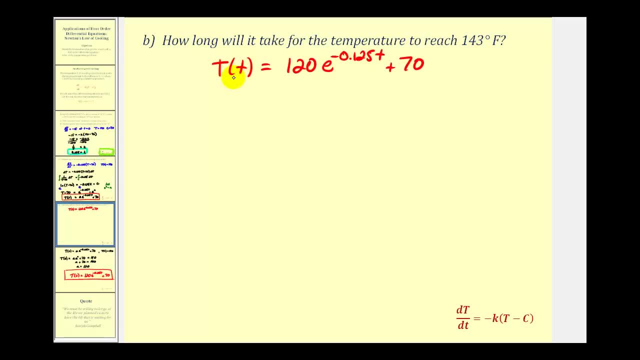 So we'll set big T of t equal to 143, and then solve for little t. So we'll subtract 70 on both sides So we'll have 73, equals 120, times e to the negative 0.125t. 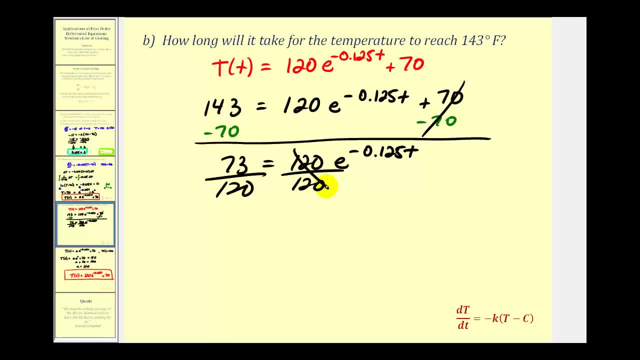 divide both sides by 120,. and now to solve for t, we'll take the natural log of both sides of the equation and then we can apply the power property of logarithms here and move this exponent and move this exponent to the front.